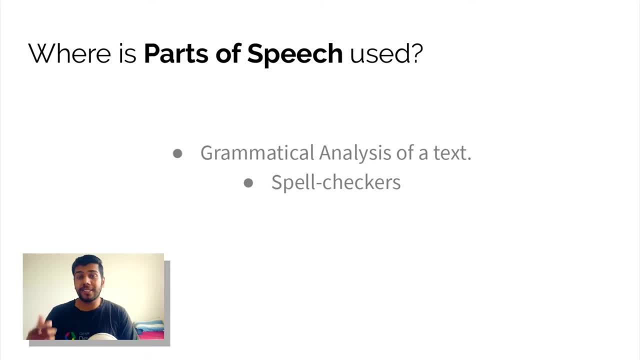 But before we go and learn about parts of speech, we need to understand what is the significance. Why are we doing it right? So parts of speech is very readily used around the natural language processing pipeline and you can easily see them in spelling checkers, in grammatical checkers. 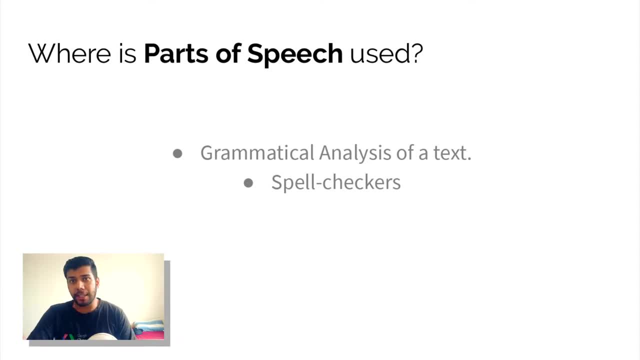 So, for example, there's a software called Grammarly and you can- you must have seen the ads For that- And it does the grammatical checking and spell checking for you Right. So there will be in the backhand parts of speech model running. 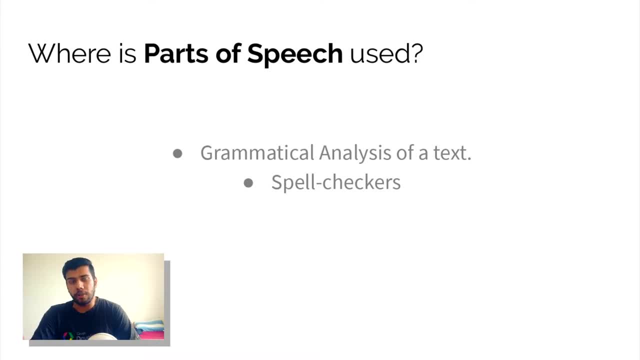 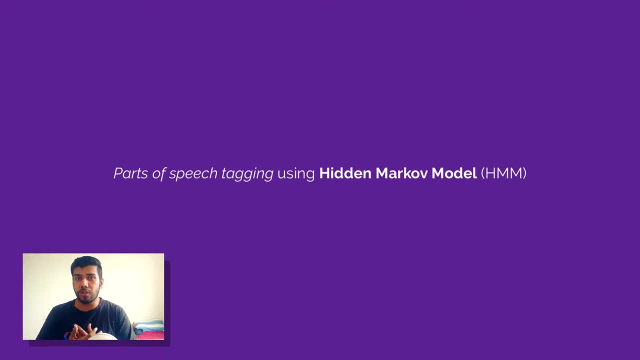 So this is just a basic example why we are doing part of speech analysis, why are trying to learn that. So we'll be going through various ways in which you can do parts of speech analysis, various ways how you can tag parts of speech in a sentence. 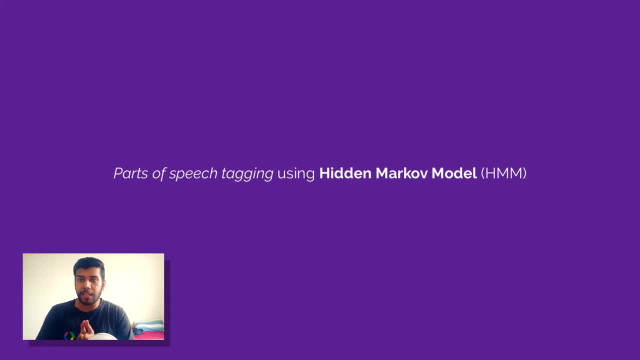 But our end goal will be to learn the state of the art model that is present right now. That is hidden model. Before I start, I would suggest that, even though you might be thinking that you need a lot of grammatical knowledge, you might think that you need, let's say, MS in English, but you don't. 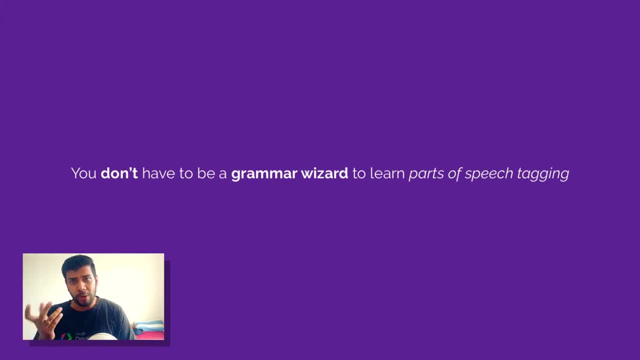 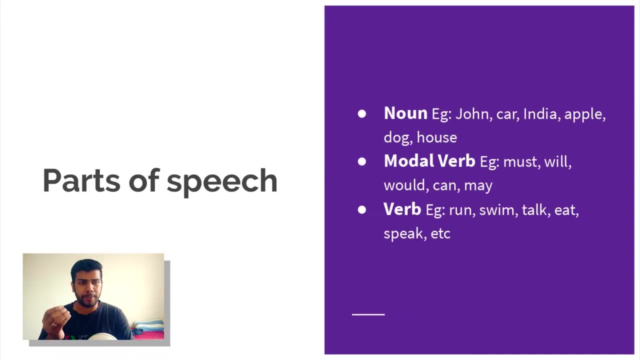 You just need to have a basic understanding about what the verb is, what a noun is, and that's it. The rest the model will take care of for you. There can be various parts of speech in a sentence, but for simplicity we'll be trying to do with just three parts of speech. 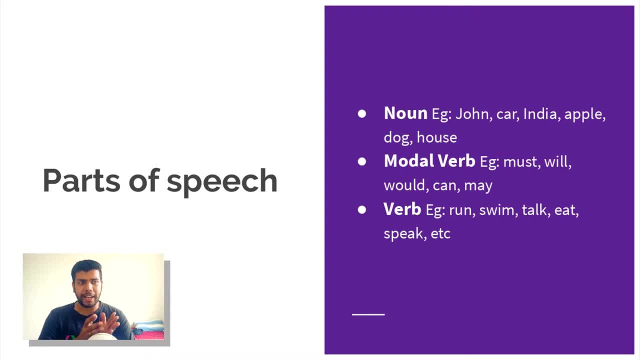 Basically nouns, Noun, which can be a name like John, car, India, apple, dog and house, just for example. Then we'll be looking for model verbs which will be must, will, can, may, would, Right. then we'll be looking for verbs. 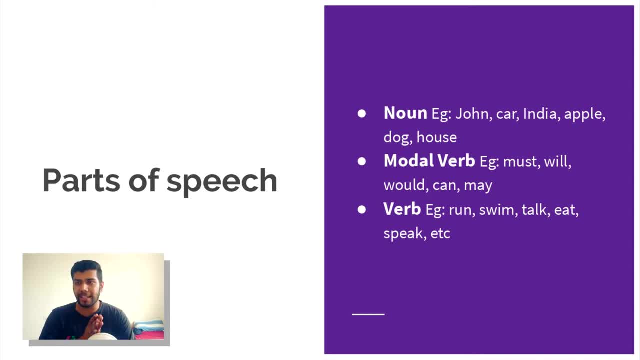 Verbs are basically actions like running, swimming, talk, eat, speak, etc. So we'll be looking for these three parts of speech in a sentence and try to guess what each and every word has the category in the grammatical space. Let's say there are three friends: Mary, Jane and Will. 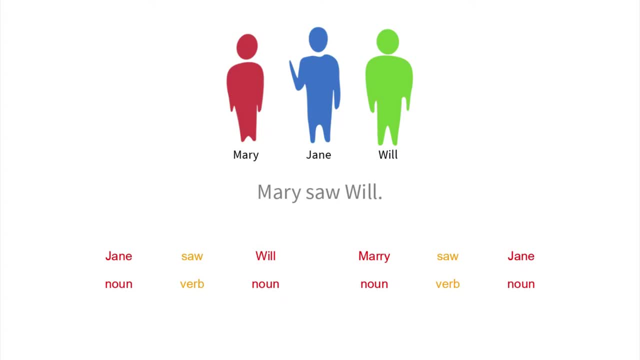 And we want to tag the sentence Mary saw Will And since we need some label data, we have label data as follows: Jane saw Will, Jane is a noun, saw is a verb and will is obviously a noun, since Will is a friend and it's the name of the person. 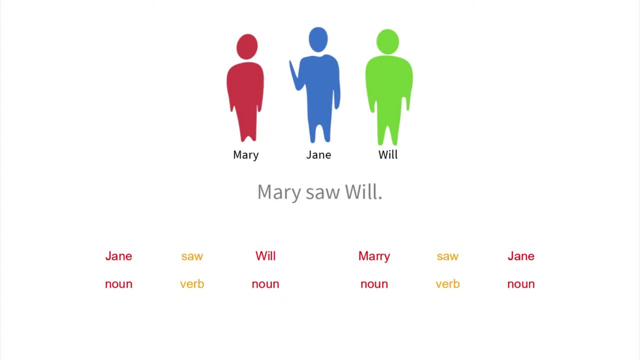 And we also have Mary saw Jane. So we'll be using our label data to predict each and every word's category in Mary saw Will. So our first algorithm is very naive and very easy. You know which will do: We'll be trying to use the most common part of speech associated with a word. 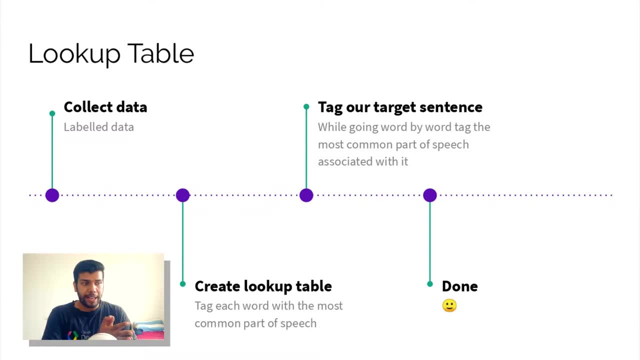 So first, what we'll be doing is we'll be collecting the data which we already have. Then we'll be creating a lookup table. So what is a lookup table? We'll be tagging each word with the most common part of speech that is associated with that word. 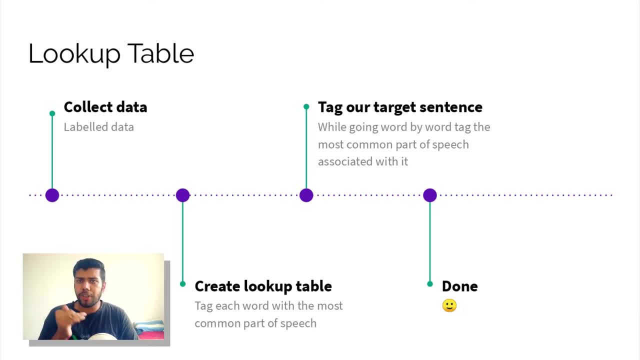 Then we'll be taking a target sentence, basically the sentence that we are trying to figure out the part of speech for, And we'll be going word by word and tagging the most common part of speech associated with it And that's it. So, if we go with our data, so we have: Jane saw Will. Mary saw Jane. 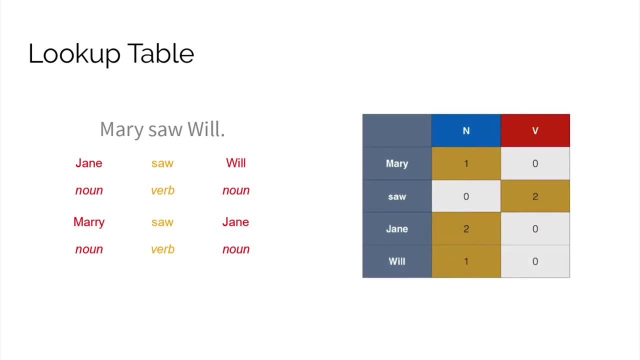 And in that we can see Mary occurred once and that once it was a noun And saw occurred twice, each and every time it was a verb. Jane occurred twice, each and every time it was a noun. And Will occurred once, and it was a noun as well. 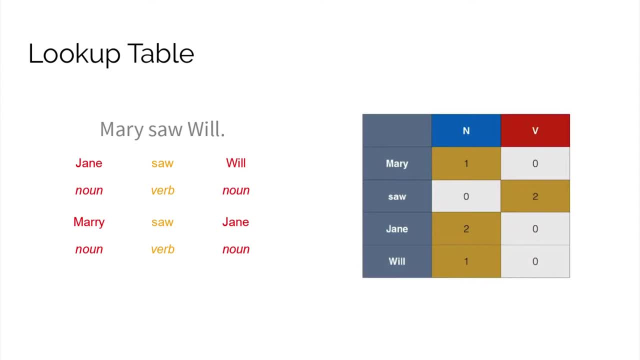 So looking at the lookup table now, we can find for each and every word the most common occurring part of speech. So first we go for Mary. So Mary almost each and every time. so most commonly it occurs as a noun. So we'll say that Mary is a noun. 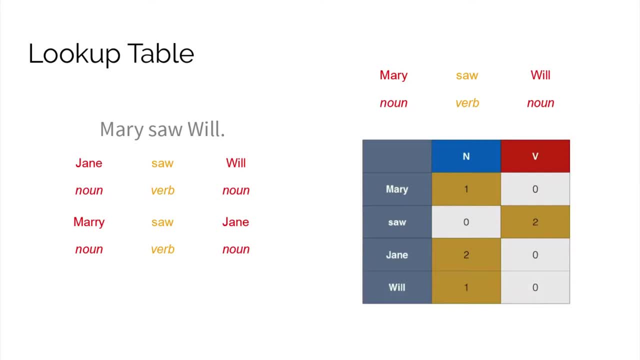 Saw always occurs as a verb, So we'll say saw is a verb And Will always occur as a noun, So we'll say Will is also a noun. So this seems pretty straightforward that we have to just go word by word and look for the most commonly occurring part of speech. 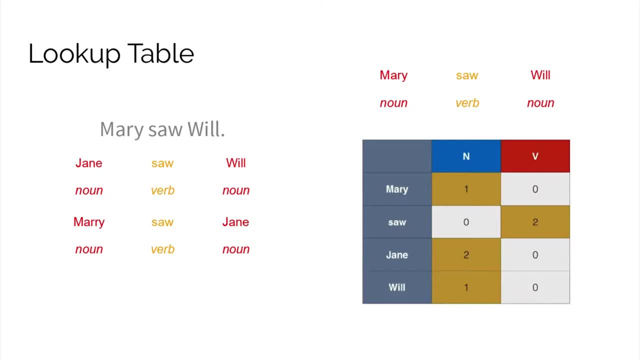 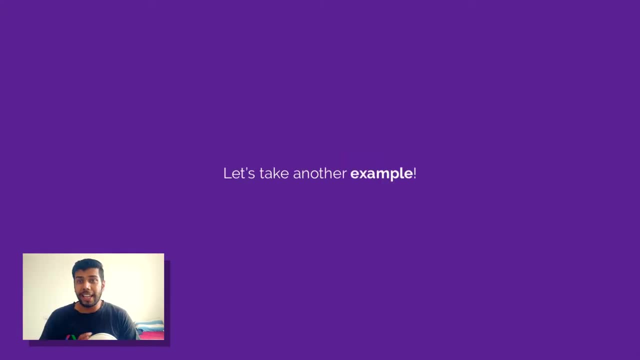 But this is way too simple, don't you think? And if I say this won't work all the time, can you think why? Let's take another example. So again, we have three friends: Mary, Jane and Will. But now our label data has broadened. 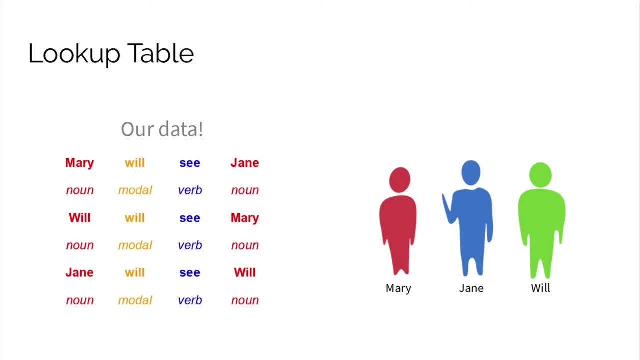 And we have Mary will see Jane, in which Will is a model verb. Then we have Will will see Mary, in which the first Will, since it is the name of the person, is a noun. Then we have Will, which is a model verb. 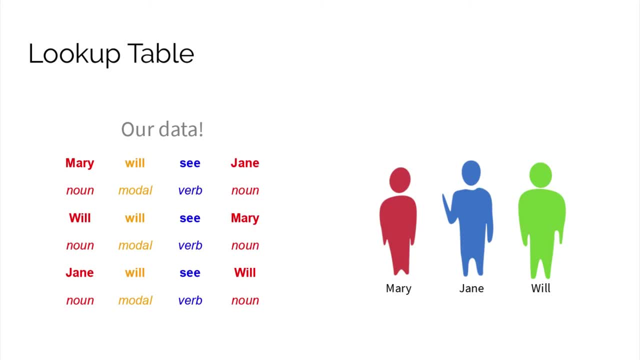 And See is a verb, Mary is a noun And we also have Jane will see Will And this time we'll be trying to predict the parts of speech tags for Mary will see Will. And first of all, obviously, we'll be creating the lookup table. 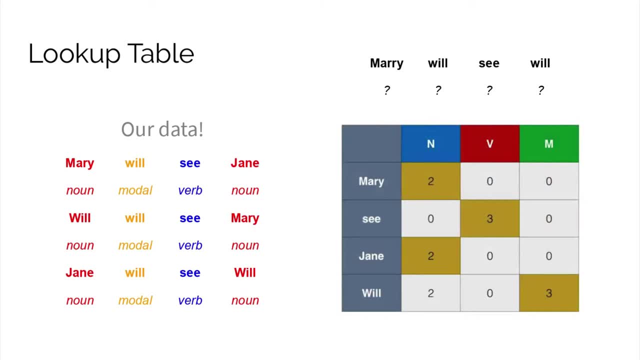 So Mary occurred twice, And each and every time it's a noun. See occurs thrice. Each and every time it's a verb. Jane occurred twice. Each and every time it's a noun. Will occurred five times, And it was a noun as well as a model verb. 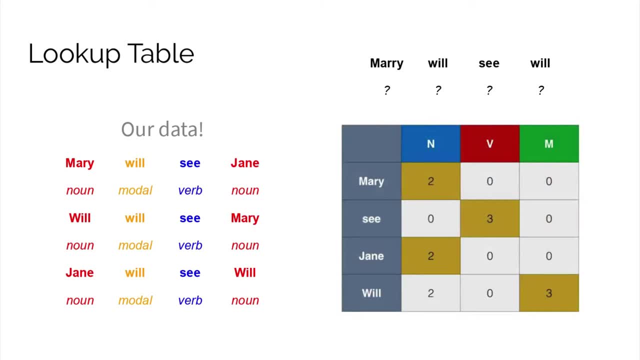 But most commonly it occurred as a model verb. Now let's go and tag each and every word. So, Mary is pretty straightforward: It always occurs as a noun. Will is a model verb, because Will most commonly occurs as a model verb. See is a verb. 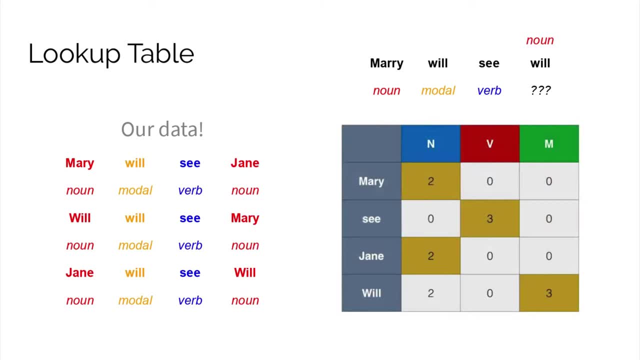 It always occurs as a verb. But now we come to the name of the person: Will, But it's a noun, But our lookup table says it's a model verb. Can you see the problem That for each and every word it will always give the same answer? 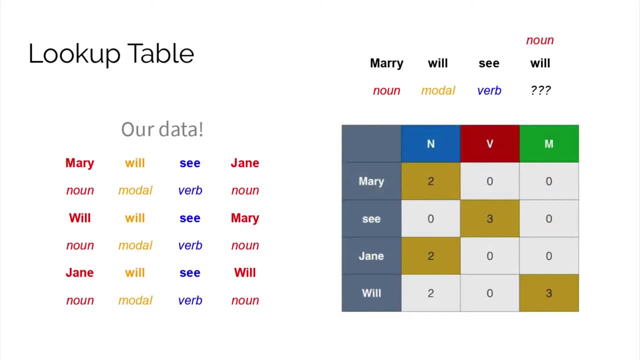 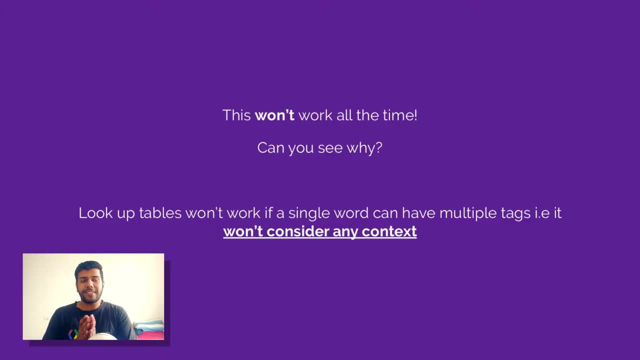 For every particular unique word, you'll always get the same answer, Be it that the context for that verb might be different. So now we can answer why this won't work each and every time. Lookup table with just a single word does not consider the context that the word is used in. 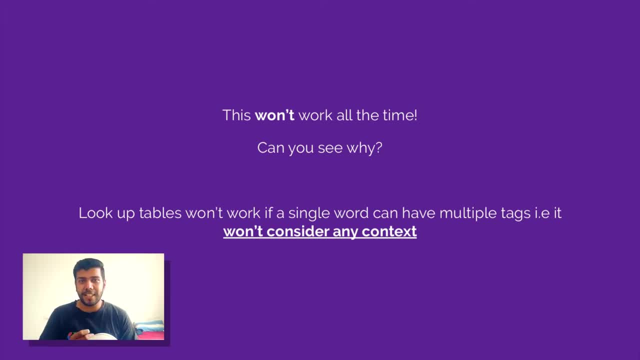 So, as a problem-stater in broadens and almost each and every time in real world, you'll be considering the context, because most of our sentences are based on context. So how can we consider the context? One of the ways in which we can consider the context: 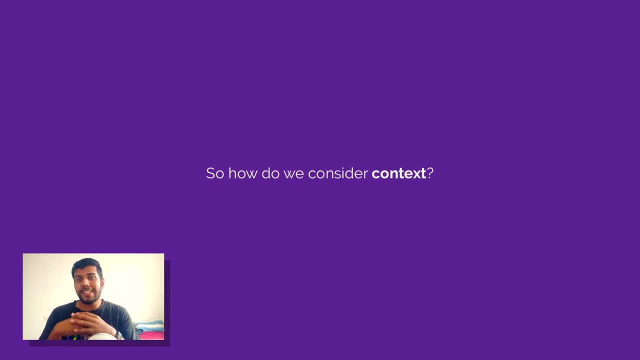 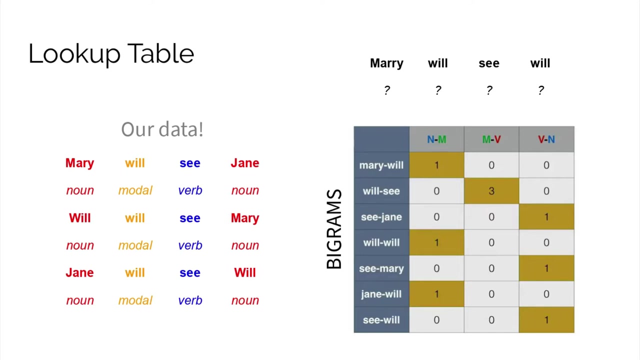 is basically using bigrams, In which we take into consideration how the word was used, Basically looking at each and every word's neighbor. So, each and every time looking for the neighbor, we'll be creating a lookup table again And we can see Mary will occurred once. 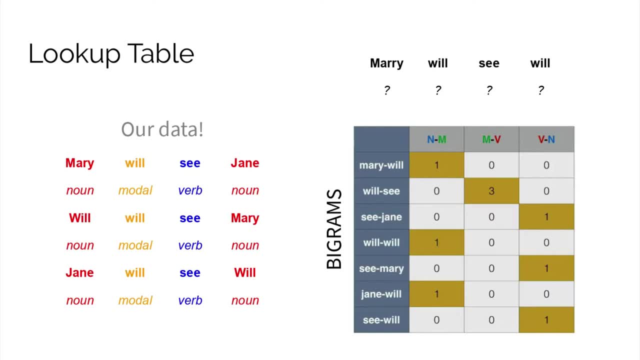 And at that time it was noun followed by a model verb, As in the same way will see occurred thrice, And each and every time it was model verb followed by a model verb, So on and so forth. we can create a lookup table. 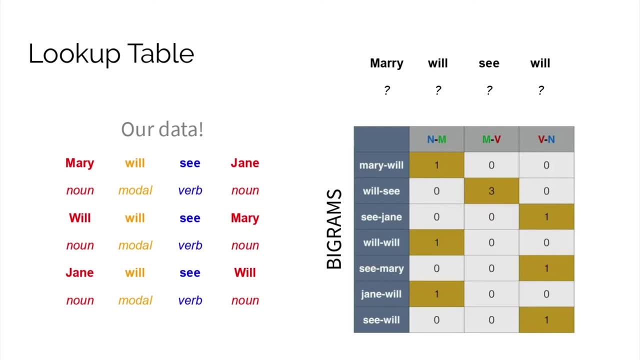 Now let's move on to a sentence. So the first word that we'll be tagging we'll be using the previous lookup table that we already created. So, Mary, almost each and every time it occurred as a noun, So we'll tag it as a noun. 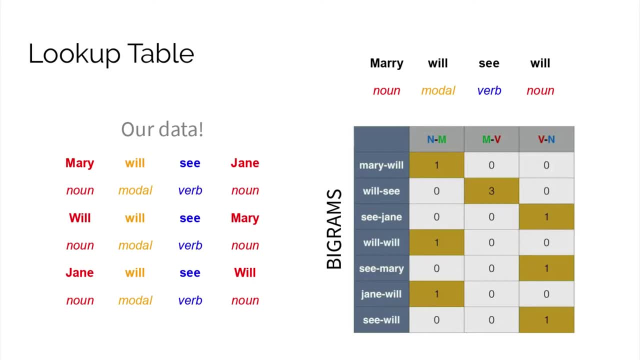 So for each and every following word, we'll be using this lookup table And we'll be considering how the word was followed by and basically considering the neighbors and the context that the word was used in. So if we go for will Mary will occurred once. 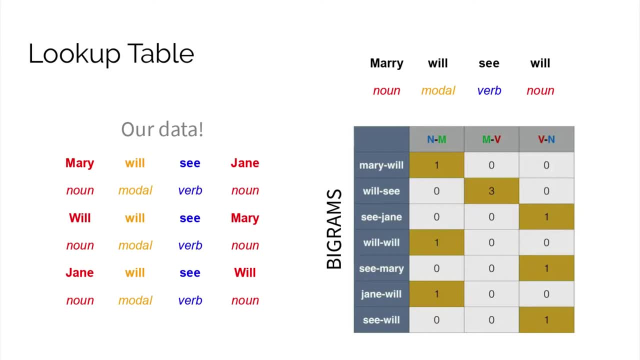 And in that time it was noun followed by a model verb. So we'll say that will is a model verb. So in the same way we'll go on and tag all the words So will see occurred thrice, And then the will will be have to consider that that will was a model verb. 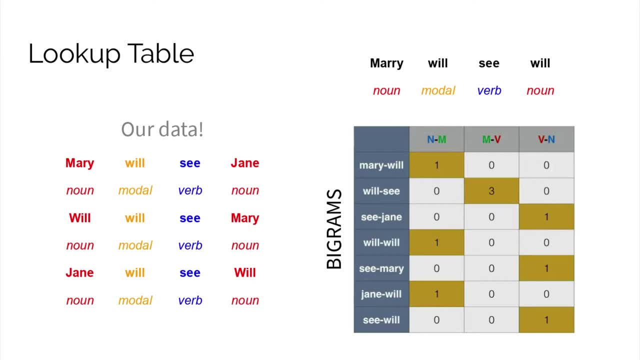 It occurred thrice And at that time see was considered as a verb. Then see will only occurred once in which the see was a verb And then will was a noun. So now we have tagged Mary will see will correctly And we have also considered the neighbors. 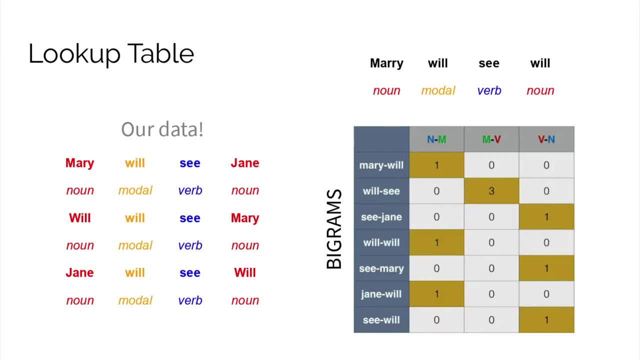 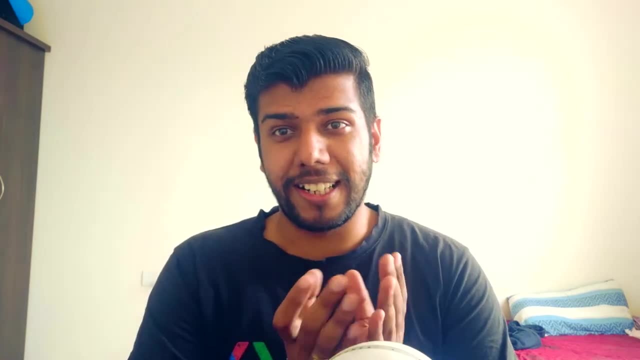 and thus the context in which the word was used. So we have correctly labeled one will as a model verb and the other will as a noun, which is correct. Now, this seems the perfect algorithm, But if I say that this algorithm also has some problems, right? 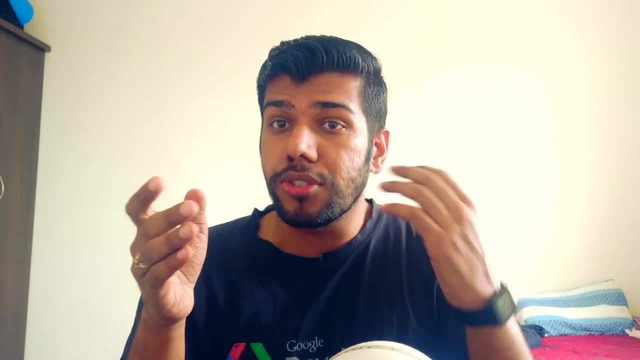 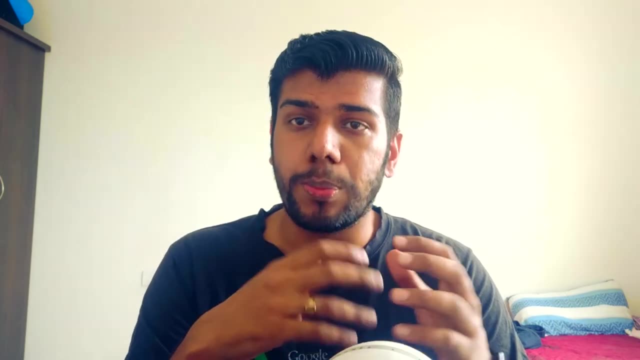 But you can even extrapolate on that. Let's say, instead of using the bigrams, you use trigrams. You can even experiment in using the both lookup tables for one word, as well as bigrams, trigrams, basically ngrams- and find out the perfect match that works for your test data. 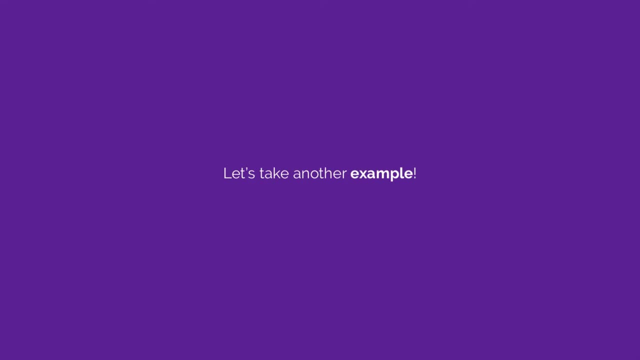 as well as your training data right. You can even use the previous table as well as this table in conjunction, so that one table corrects if there is a wrong prediction made by the other table. So now, since you are able to use ngrams and the lookup tables pretty efficiently, 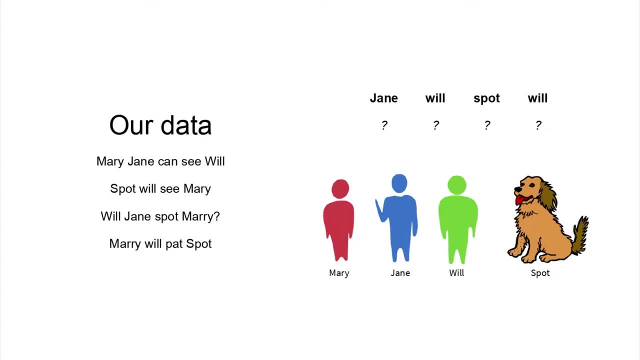 let's spice up the problem a little bit. So already we had three friends: Mary, Jane and Will. But now there is another person in the mix Spot And our data, our label data, is containing Mary Jane can see Will. 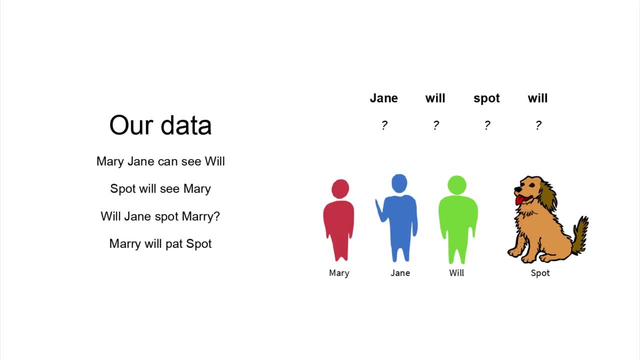 Spot will see Mary Will, Jane spot Mary and Mary will add Spot, And the target sentence that we are trying to predict is Jane will, spot Will. So now again, we'll be creating a lookup tables. We're creating a table with bigrams. 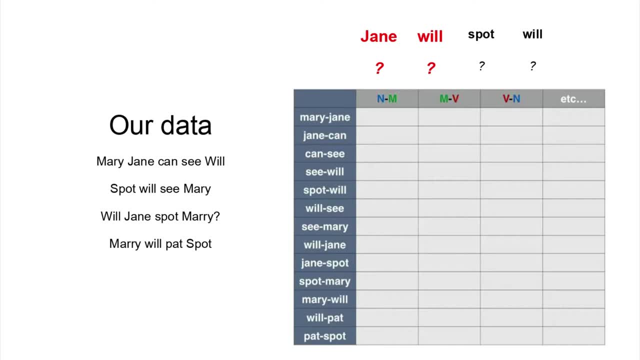 And now we have got a problem. If you see, in all the cases Jane, followed by Will, never occurs in a training data, And now we have no way of knowing what Jane and Will be if we know one of the neighbors. So wherever there is a problem, there is a solution. 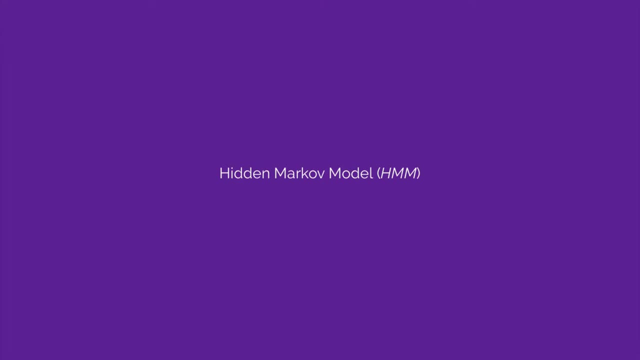 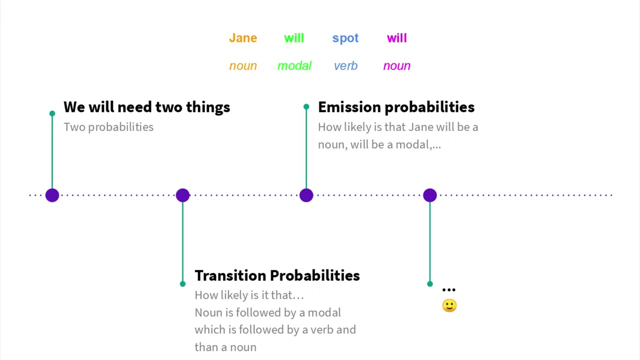 And I think this is the best time to consider the hidden Markov model. So the hidden Markov model is a probabilistic model in which we'll be considering the probabilities. So there are two probabilities that we'll be using. The first one is the transition probability. 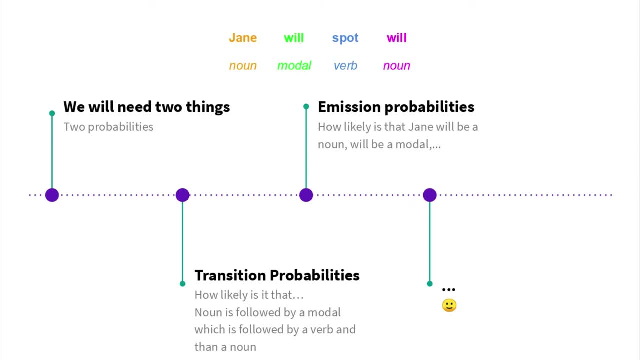 What is that? So it's: how likely is that a noun will be followed by a verb. So, basically, how likely. if Jane is a noun, the next word that occurs is also a noun, or also a model verb or also a verb right. 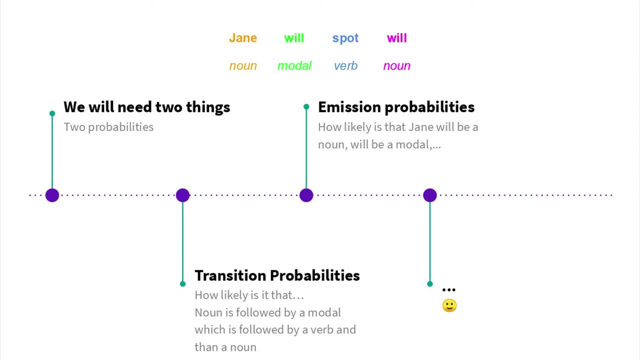 So how likely is a noun followed by a model, or how likely is a model followed by a verb, or how likely is a verb followed by a noun? The second probability that we'll be considering is the emission probabilities. So how likely is Jane will be a noun, or will it be a model, or will it be a verb? 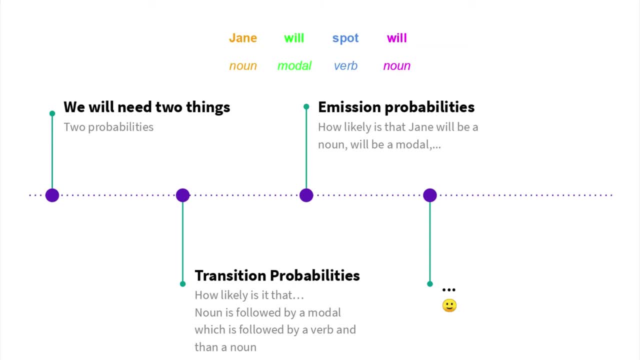 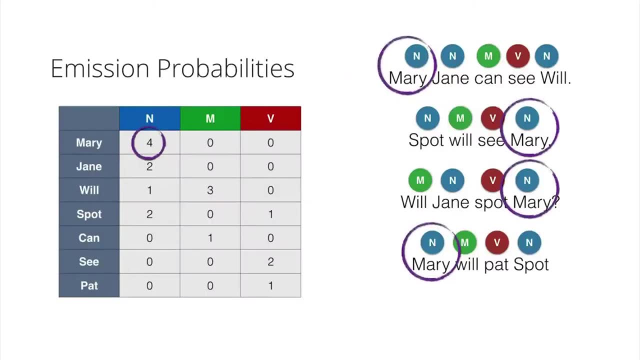 So this is emission probabilities. So, considering these two probabilities, we'll be using the hidden Markov model. So first let's work on emission probabilities. Before doing that, let's create a simple lookup table in which we just plot out how many times Mary was stated as a noun, as a model verb or as a verb. 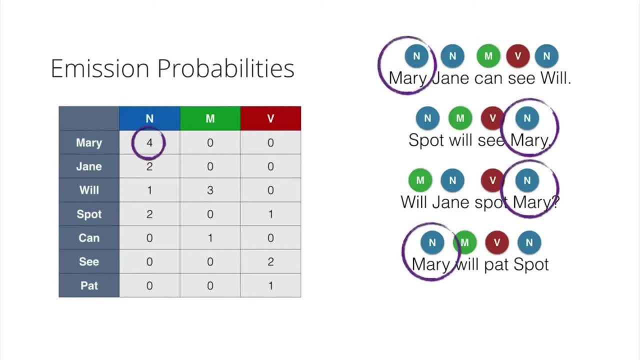 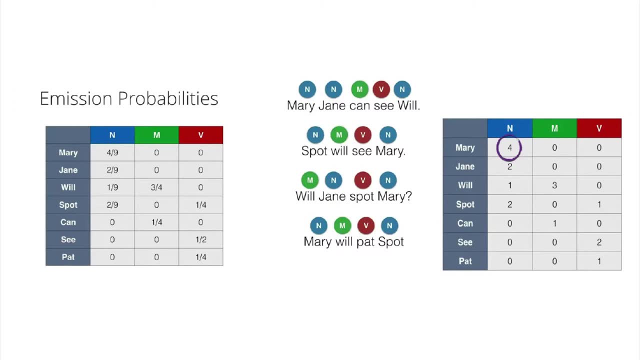 And we can see. Mary occurred four times and each and every time it was a noun. Then we go for Jane. Jane occurred twice and it was a noun all the time Will occurred four times, but once it was a noun, all the other times it was a model verb. 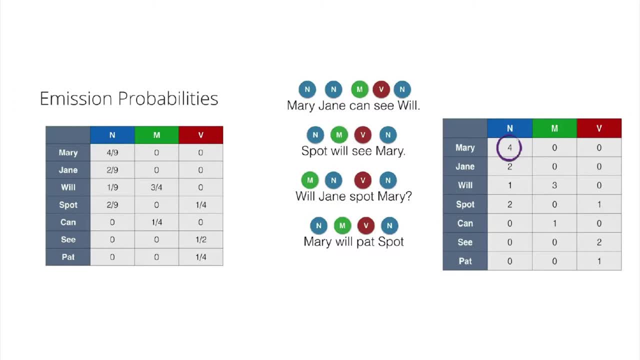 So we'll go on and do for each and every unique words. spot can see and pat. So now let's consider a possibility that Jane is a noun, Will is a model verb, Spot is a verb And again, will is a noun. 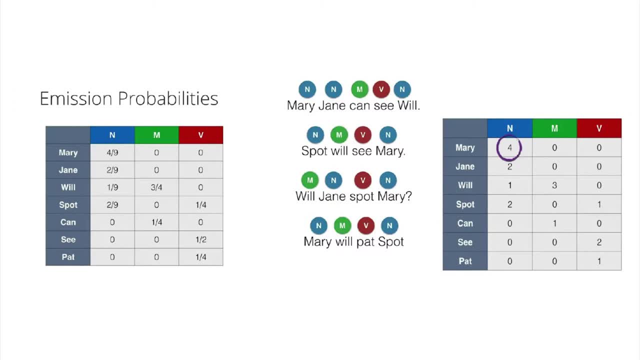 So what we'll be considering is how probable it is that if Jane is a noun, the next word- basically if it is a noun- the next word that will be occurring- will a model. So the probability that a noun will be followed by a model will be stated as the transition probability. 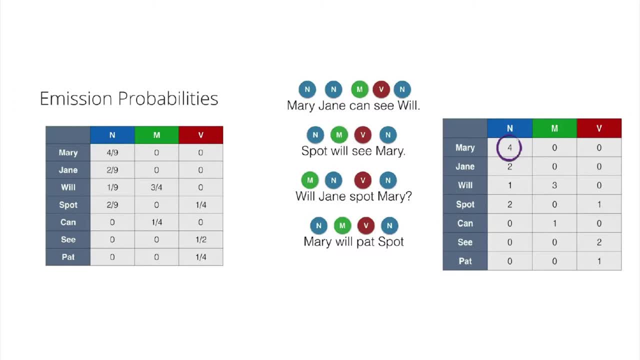 Now, how likely is that Jane will be a noun? Basically, will will be a model and spot will be a verb, And this is our emission probability. So now let's create our emission probabilities. So for Mary, we'll be stating that how probable is that, if a word is a noun, that it will be a Mary? 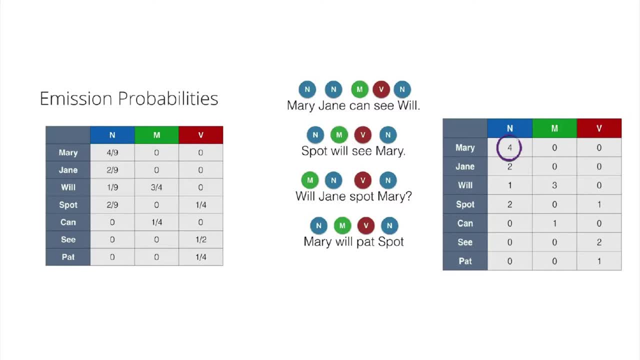 So noun occurred nine times, and out of the nine times it was four times that it was Mary. So the probability is four divided by nine, And so we go for Jane. So noun occurred nine times and it was twice that it was Jane. 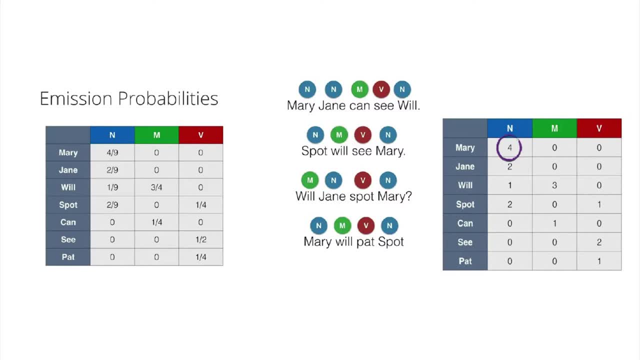 Then we go for will. Will was noun once, while the noun occurred nine times, But will was also a model verb. Model verb in total in the data occurred four times and it was three times that it was will. that was the model verb. So we go on and create the emission probabilities for each and every word. 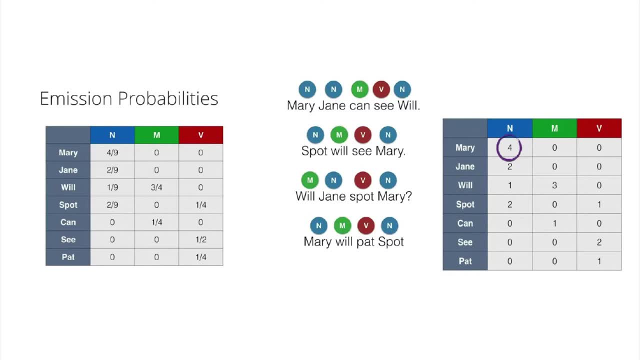 considering that a word was a specific part of speech And how probable is that that the specific word was that part of speech. So if we say that, how probable is that if a word is a noun, that it will be Jane. So we can say: if it is a noun, noun occurred nine times and only twice it was Jane. 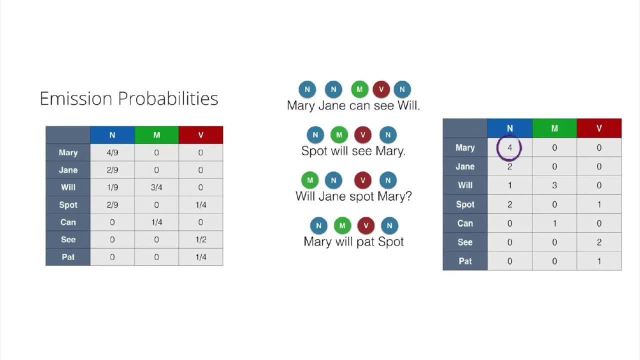 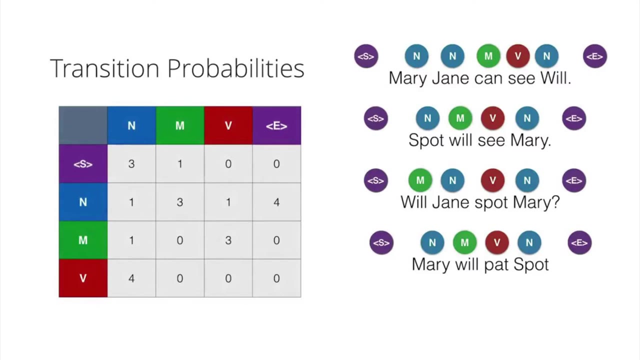 So the probability for that word to be noun and Jane will be two divided by nine. So now we move on to the second probability that we have to discuss, And that is transition probabilities. So transition probability is how likely, let's say, a noun will be followed by a noun. 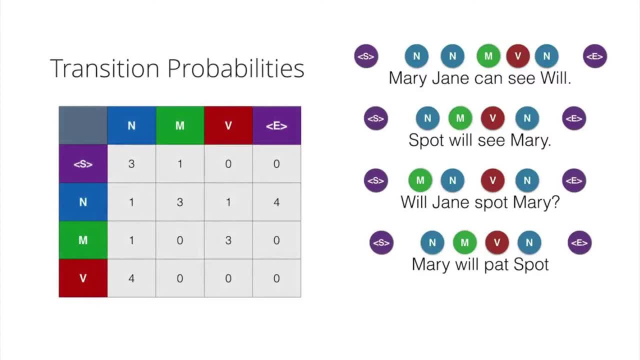 How likely is a model verb will be followed by a noun, Or how likely is a verb will be followed by a noun? Basically, how likely is one part of speech followed by the other part of speech? But to do this we first have to add starting tags and ending tags. 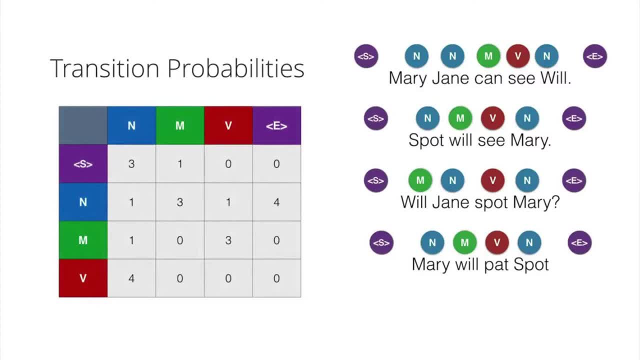 So that the first word and the last word can also be considered as followed by something. So we add tags, start tags and end tags, And we create a table in which we state how many times the start tag was followed by a noun. So start tag was followed by a noun three times. 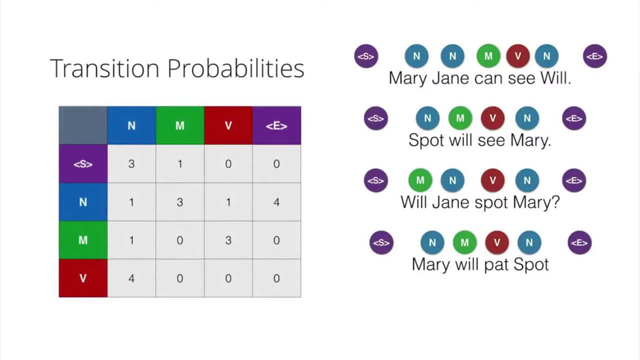 In Mary Jane. Mary Jane can see will spot. will see. Mary Mary will pat spot. So each of these times the start word was a noun, So start was followed by a noun, And only once it was that the start was followed by will. 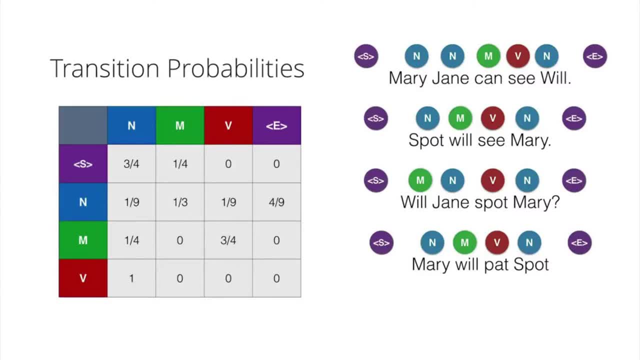 Will Jane spot Mary? Then we go with noun. How many times noun was followed by a noun? So it was just once. when we can see Mary, Jane can see will That noun was followed by a noun. We create a data in which we have how likely is that one part of speech followed by other part of speech. 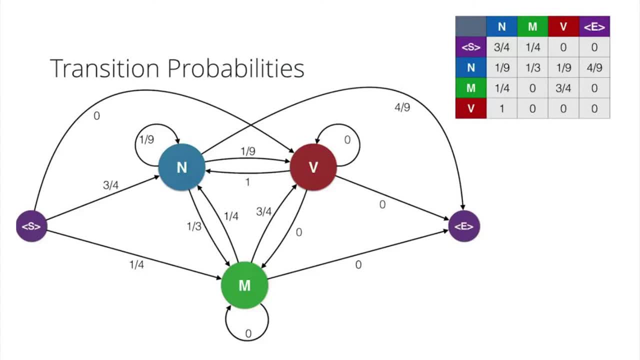 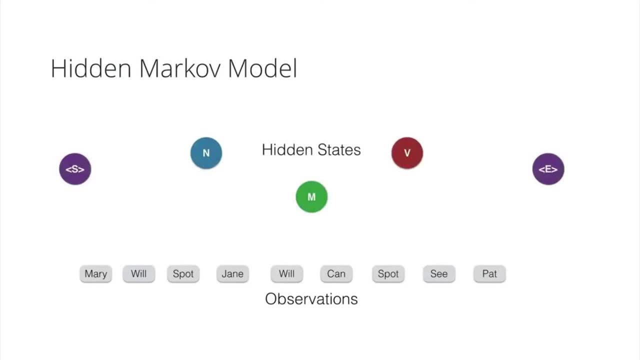 So now we combine the two probabilities, basically the two graphs that we have created, to create the hidden mark of model In which all the words Mary will spot, Jane will can spot and see Pat, Even though all the words that occurred are observations. 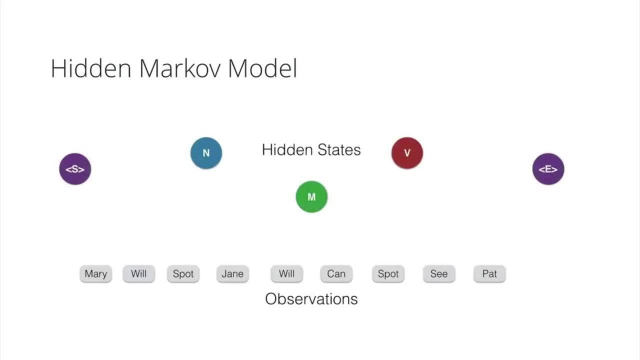 And the hidden states- basically the states that we are trying to predict- are noun model verb and the verb Observations are what we get from the sentence. the words and the hidden states are basically that we have to predict from the observations that we have. 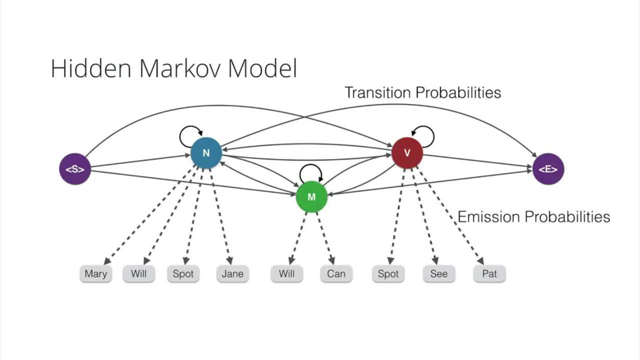 Between each and every hidden state we have transition probabilities And between the observations and the states we have emission probabilities. So how likely will be a noun followed by a model verb is a transition probability. How likely that a noun is Mary is emission probability. 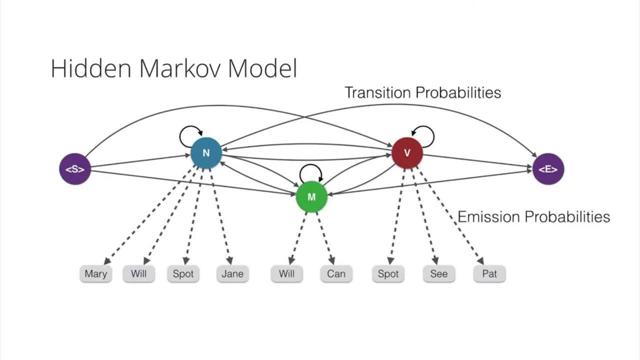 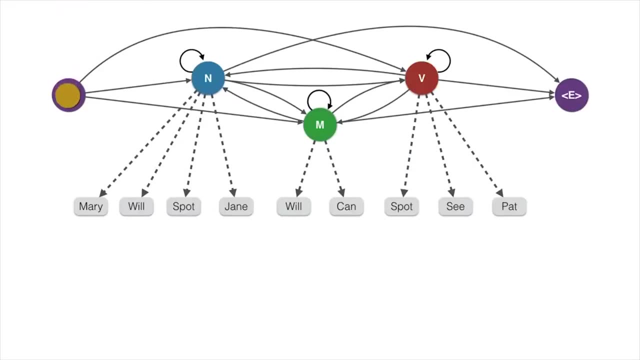 So now what we will be doing is we will be going through the hidden states with some probability. So we obviously start from the start and we go to noun. So probability that the start will be noun has some probability, which is called transition probability. After we reach noun we record the word Jane with some probability. 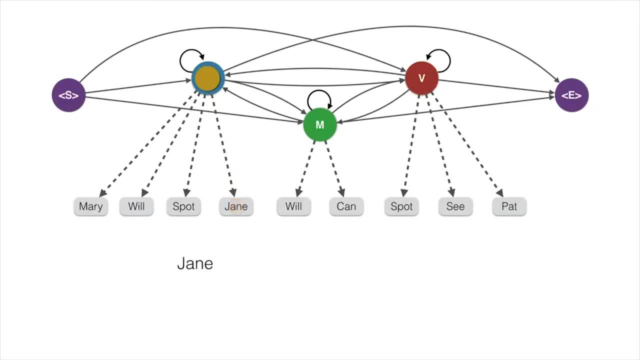 Then we go to the model verb with the transition probability and we record the word will. This is how we will be generating almost all the sentences that are possible, given our label data. So now all we have to do is record the probability that we can generate a sentence, a target sentence, with. that is, Jane will, spot will. 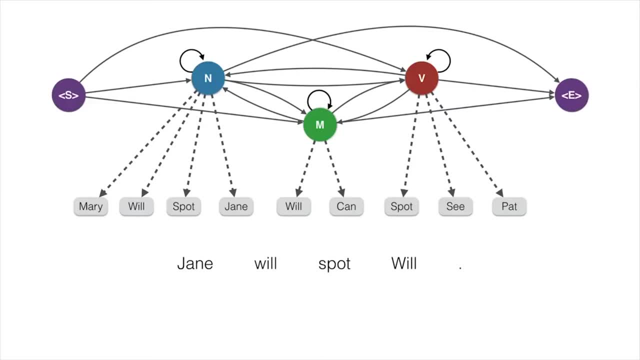 So again, we start at the starting hidden state and then we go to the noun. So the probability that the first word will be a noun has some transition probability. So now, since we have come on noun, the probability that the word at this state will be Jane has some probability. 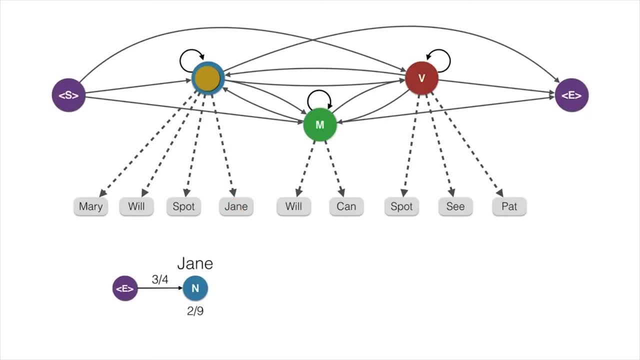 In this case it's 2 by 9 and we record that. So, till now, what we did is We started at the starting point and we recorded the probability, which is the transition probability that the next word will be a noun, Which was 3 of a quarters. 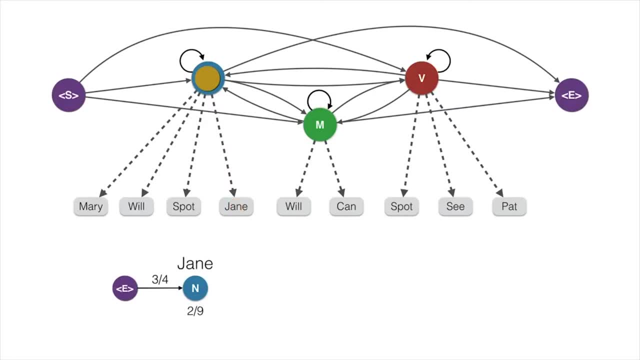 Then we recorded the probability that that noun will be Jane. That is the emission probability, which is 2 by 9.. Now we go from noun to model verb, And now we record again the transition probability that noun will be followed by a model verb. 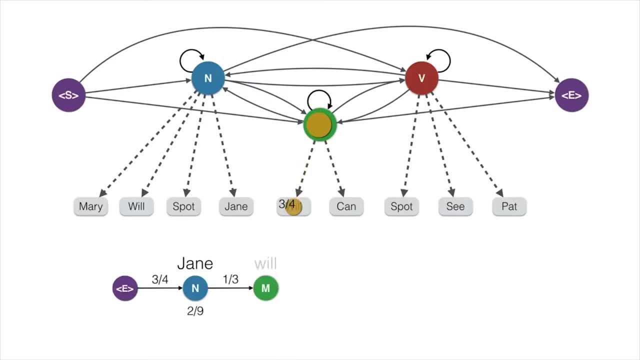 Which is 3 by 9 or 1 by 3.. Then we record the probability that the model verb will be will, Which is 3 by 4.. So we go on from model verb to verb, Record the probability. What is the probability that that verb will be spot? 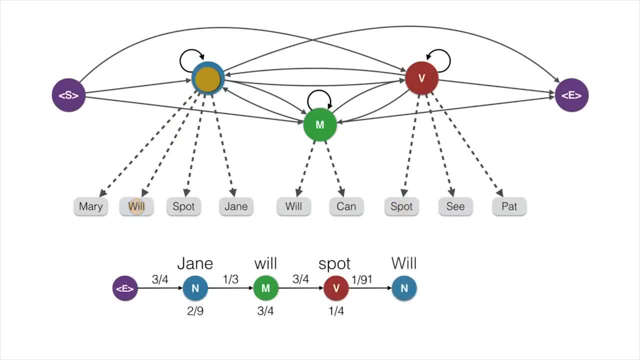 Which is the emission probability. Then we go from verb to noun, Noun to the end of the sentence. So now we. So what we do is now, since we have all the probabilities, We multiply them, Which is 0.003858. 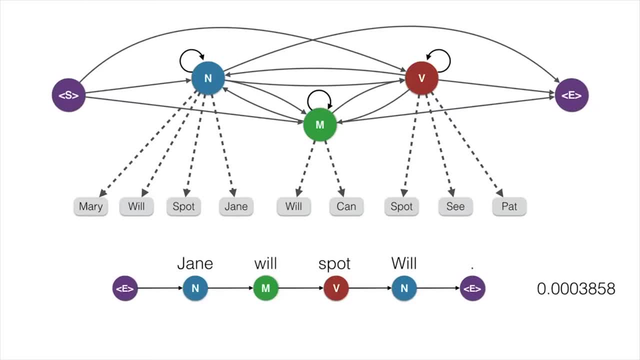 So now you might be wondering: why did we multiply them, Since each and every probability is independent of all the other events. So since how likely that the starting word is a noun Has absolutely no effect on how likely is that noun will be followed by a model verb, 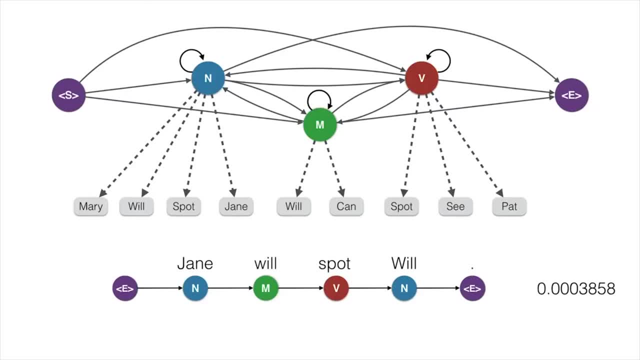 And that does not have any effect that how likely that model verb will be will. You might also have a question that the probability that we got is very, very small And you obviously know the answer that we got here is correct. So how can we say with confidence that we got the correct answer? 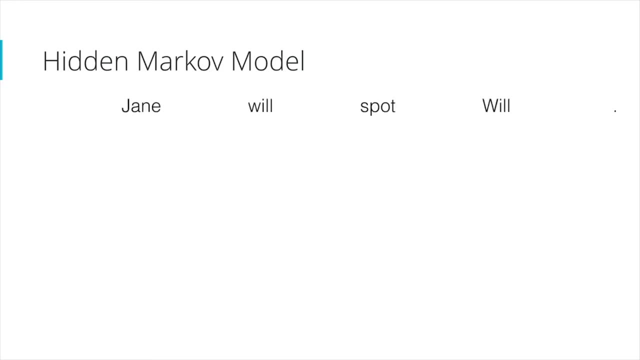 The thing is that we have to consider this probability Relative to all the other states that we considered and the probabilities that we got. Let's say, we consider the hidden states for each and every observation as noun. The probability for that is 0.000000. 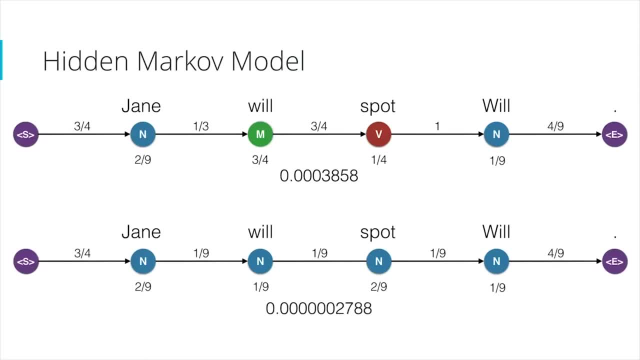 0.000000.. 0.0000002788. Which, if we compare with the probability that we got earlier, is extremely small. So, basically, we can compare the probabilities for each and every observation and hidden state combo That we create and pick up the probability that is the highest. 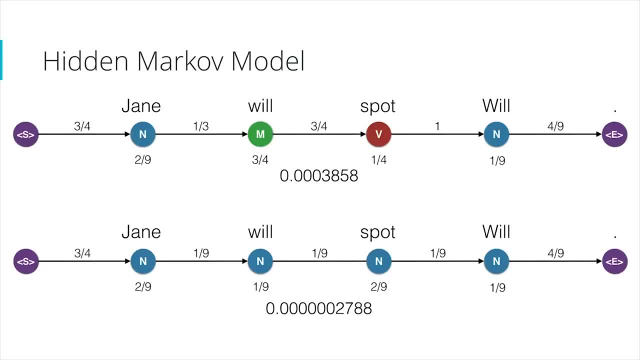 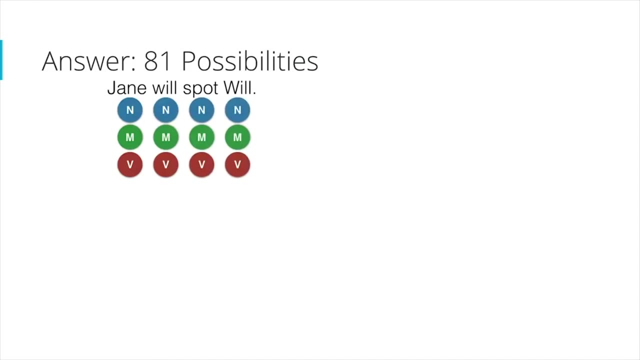 So how likely that that sentence- we have that set of hidden states- Will take the best possible outcome that we can predict. But now here, can you guess how many probabilities that you will be comparing So to calculate that we can say that for each and every observation. 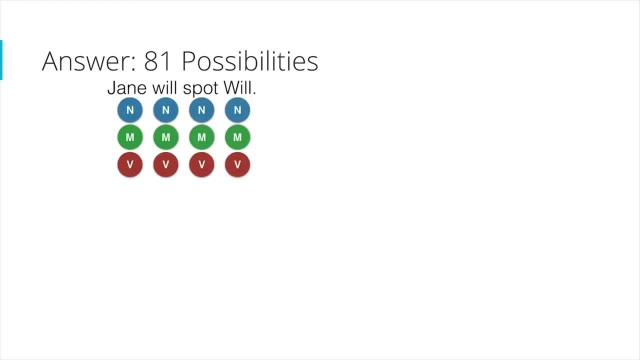 There can be three hidden states associated with it, Which is basically noun model, verb and verb. So Jane can be noun model, verb or a verb. Will can be noun model or a verb. Spot can be noun model or a verb. 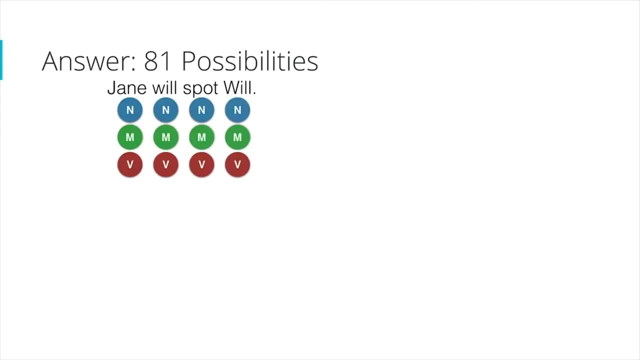 And will can also be noun, model or a verb. So each and every state has three hidden states That can be associated with it. So the answer of all the possibilities, or all the paths or the probabilities that we have to compare, Is 3 to the power of 4.. 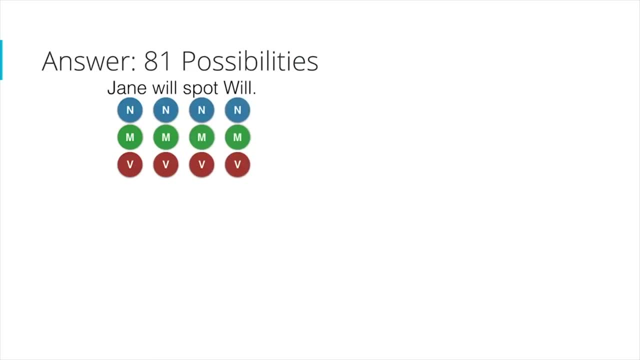 Which is 81. And how will be calculating the total probability for each and every possibility? The 81 possibilities that we just calculated is Will be taking all the transition probabilities that a word, The starting word, is a noun and that word is followed by a model verb.